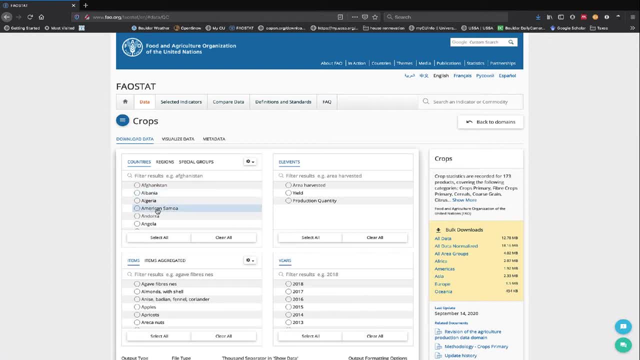 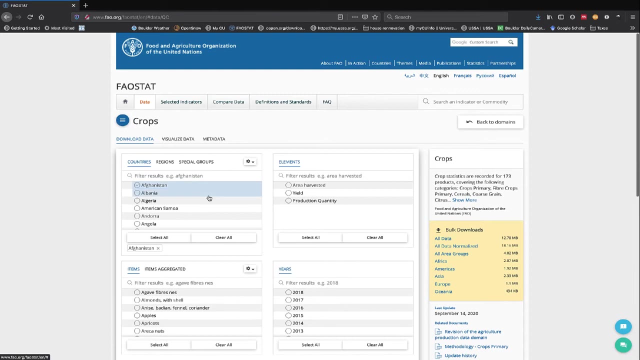 all the other data, if you ever want to get something else Right. so you have upper left countries, upper right, the data type that you're going to look at, lower left the crop types and the lower right are the years. So I'm just going to grab a couple countries. Let's just take 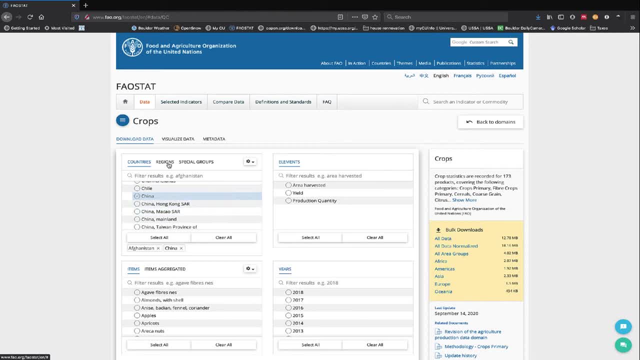 China and China. You can take as many as you want, or you can do regions including the world or North America, or you can do it by economic groups. That's what special group is, And then we're going to go over here to elements Area. harvested is the total area in the country. 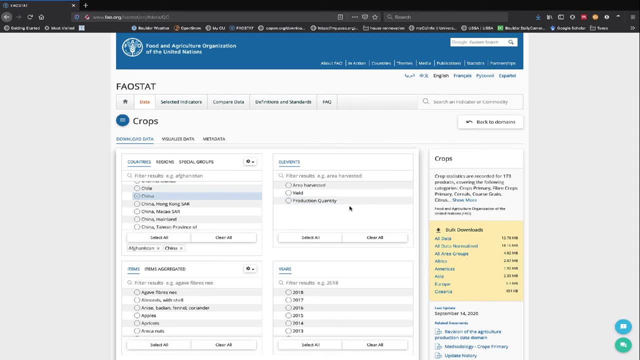 that is under a crop. Production quantity is the total quantity produced in the country. Yield is what we want, which is going to be production per unit area, So that's the one I'm going to pick. On the lower left you've got a lot of different things, So aggregated items are going to be like: 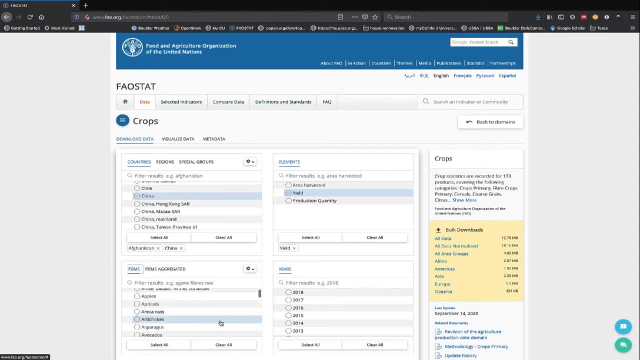 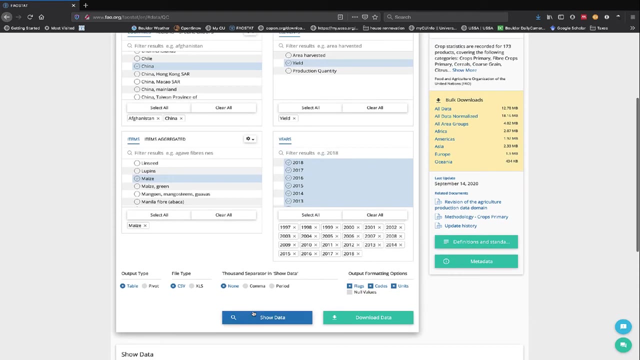 all the cereal crops or all the citrus fruit. We can go in and actually just look for maize for this exercise. Maize is the same thing as corn. Grab that and take all the data we can get. Now you have a couple different options for export down here. 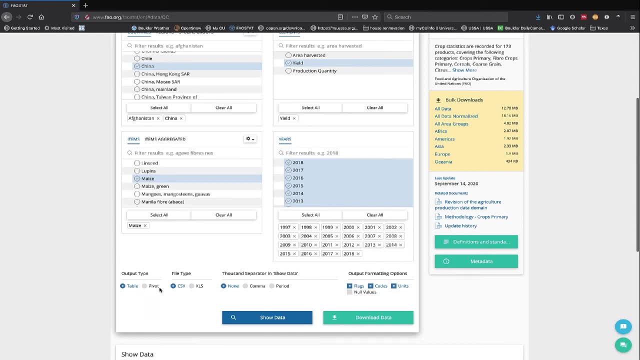 You can see them here: Table pivot, which is an inverted version of a table comma delimited text file, excel file is an inverted version of a table comma delimited text file, and so on. So if you want to see whether or not there are data for the countries you picked, 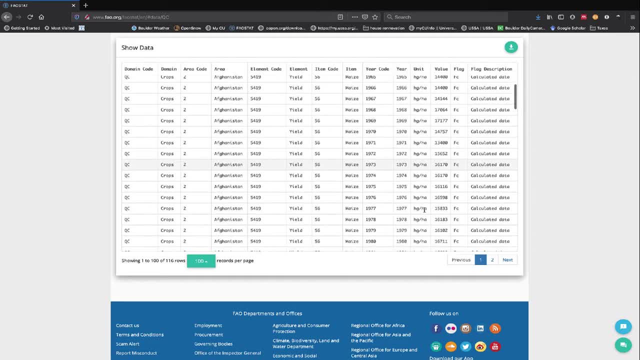 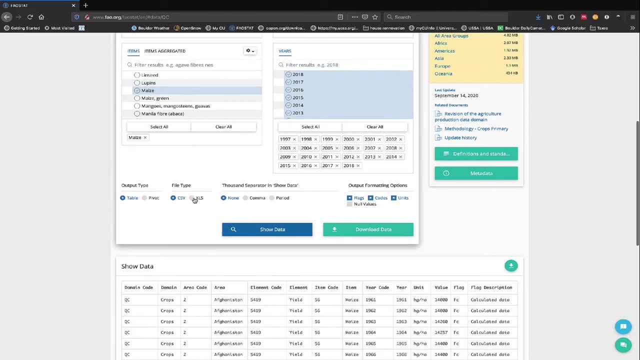 you can just do show data and it'll show you right here right below. Now you could copy and paste this, but FAO makes it really easy. So if you do table, take the XLS format and you download the data. I'm going to open that with Excel. 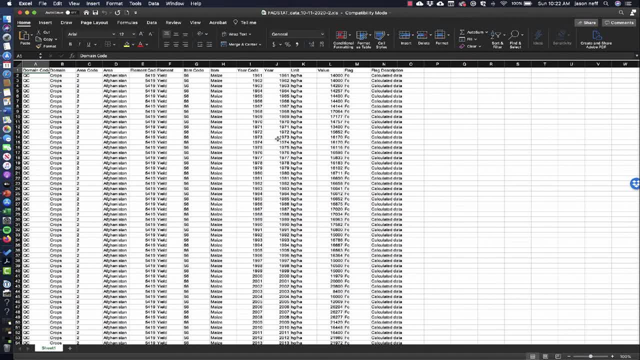 All right, I have the data in front of me Now. there's a bunch of extra information Here that you probably are not going to want, but you have your country in the column D: Afghanistan or China, the two that I picked. You're not going to worry about element code. 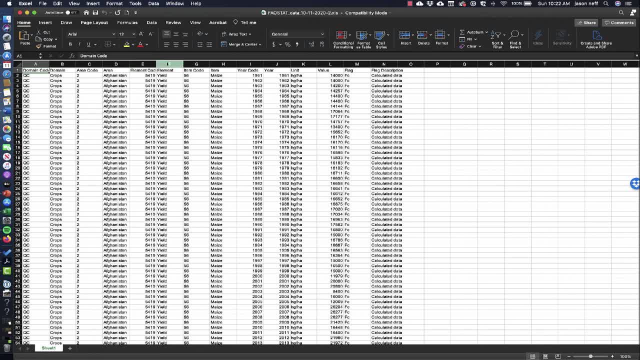 It means something to someone, but probably not to you. Just double check that you got yield. double check that you got maize here, and then you've got years done two different ways. So you only need one of those. You have the units, Just make sure you know what those are. 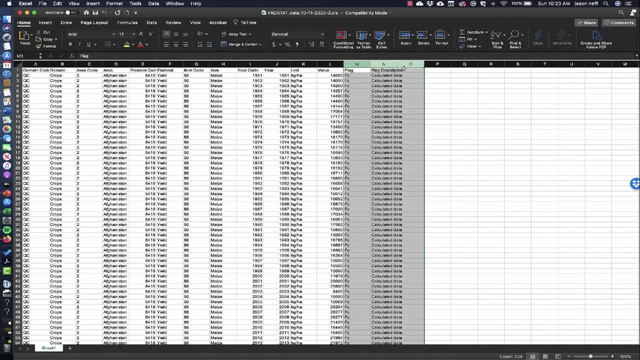 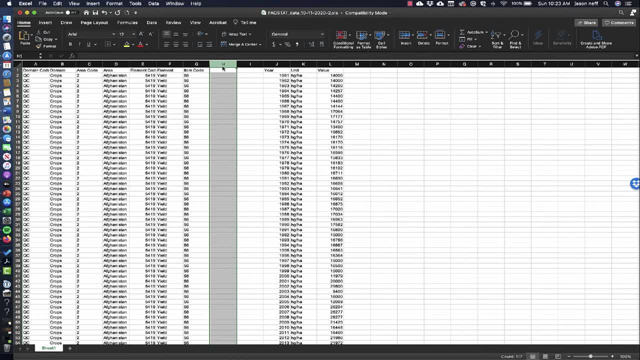 And then you have the value. So what I would tend to do would be clean up all the things that you don't need. Don't need two years. You already know that you're looking at maize. That doesn't really matter, You already know that you're looking. 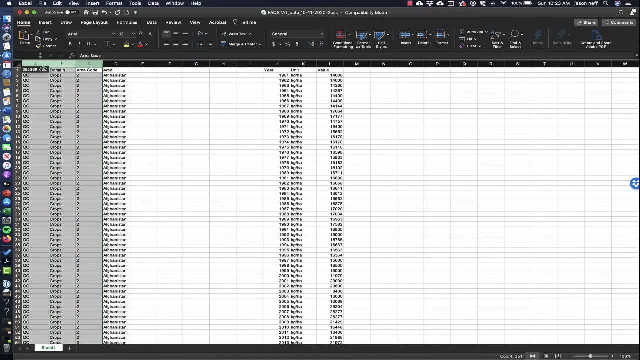 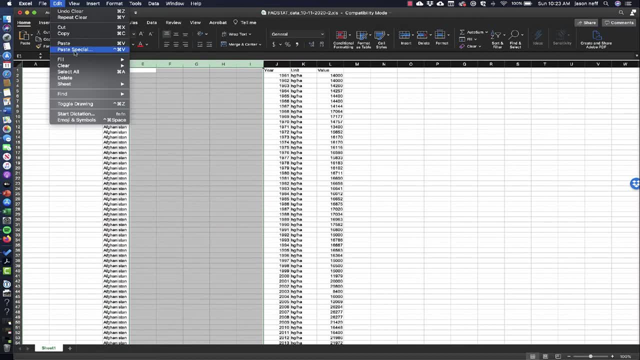 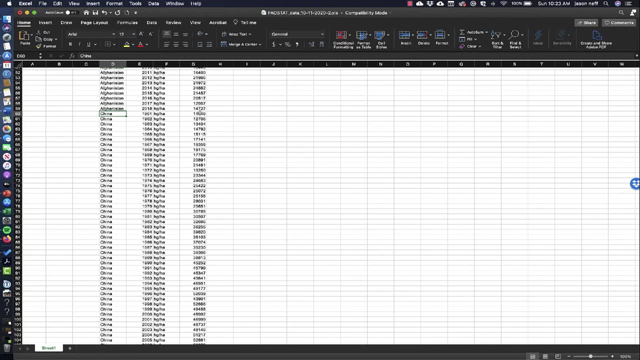 at yields. You can probably get rid of all this, And all of that's not really that useful. And you've got Afghanistan, You've got the years, And now I'm just going to clean stuff up a little bit. Delete the columns, And FAO always stacks the data like this, So you have to clean that. 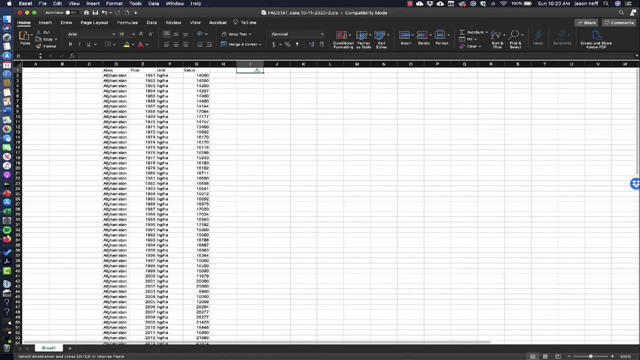 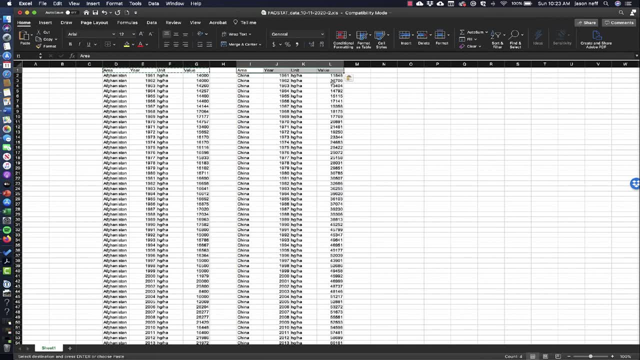 Depending how you want to look at it. probably the easiest thing is to just move it here. Make sure you're tracking what you do And from this point on you can actually do the analysis you need to do So. in prior work in this class, we've already gone through how you convert units. 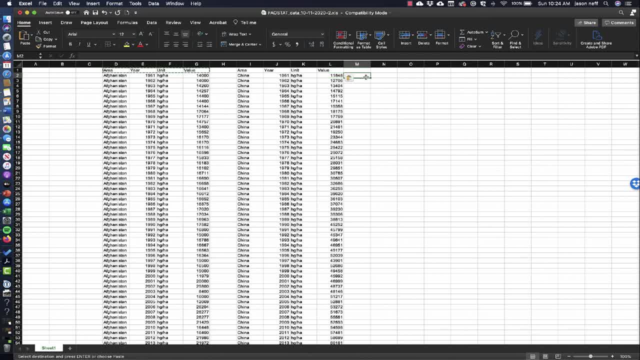 So if you want to change this from hectogram to hectare, you can do a unit conversion here. whatever that might be, times a thousand times that particular cell will give you a new number. So I would suggest you do something like that. 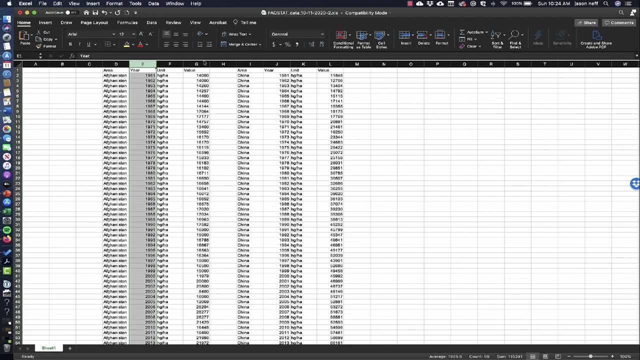 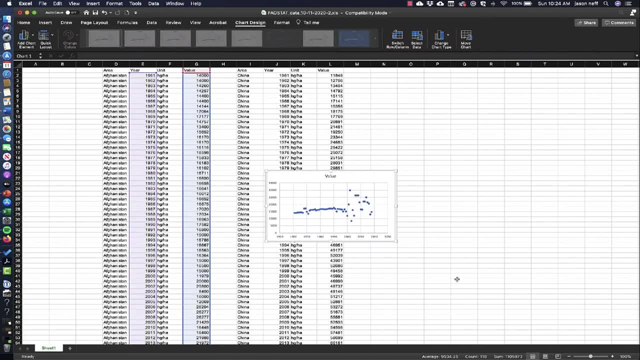 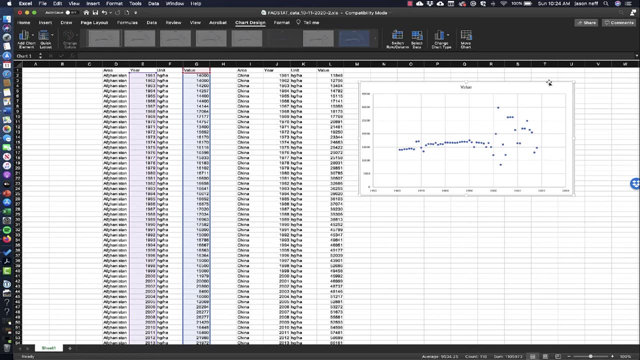 Once you're ready, you can graph the resulting data. So you have something here you can look at. Some crops are going to have big trends, Some are not. So when you go through this exercise, if you want to be with clear trends, then just look at it beforehand. You can always switch countries if you want to do. 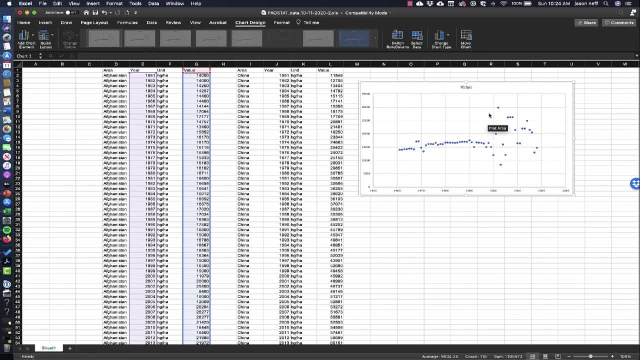 that Other countries will not. Afghanistan, you can see, goes up and down a lot here from 2000 to 2020.. That is because of war and conflict, right. So production sometimes represents real world changes. Sometimes there are errors in data. In many countries you will see a broad trend In. 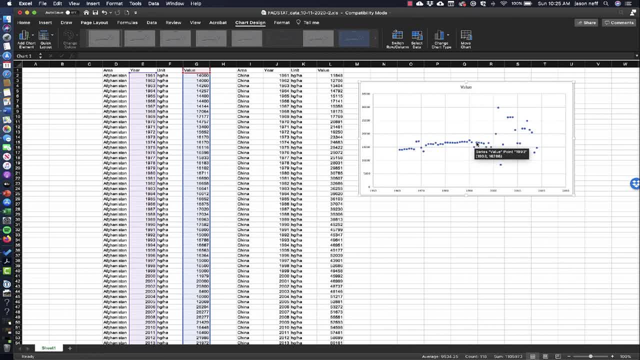 fact, in Afghanistan you see a slow upward trend as you go from 1960 to 2000.. So just have a look at your data. Everything you're going to do from here on out is like prior assignments, Fit, a linear fit to the data. That's a right click. add trend line linear. show the equation, show the. 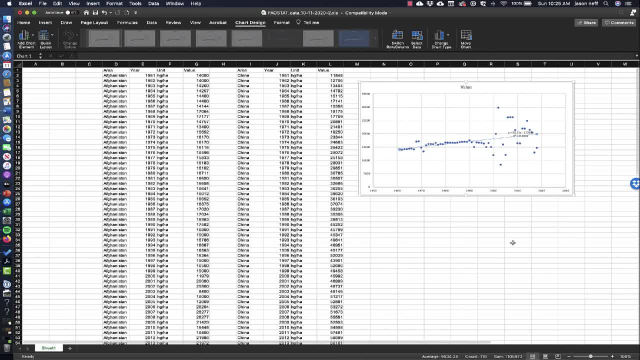 R-squared and you're off and running. So once you get going, just make sure you're doing the right thing. Just make sure you're doing the right thing. Just make sure you're doing the right thing. Make sure you're paying attention to your data. Make sure you're doing the unit conversions. 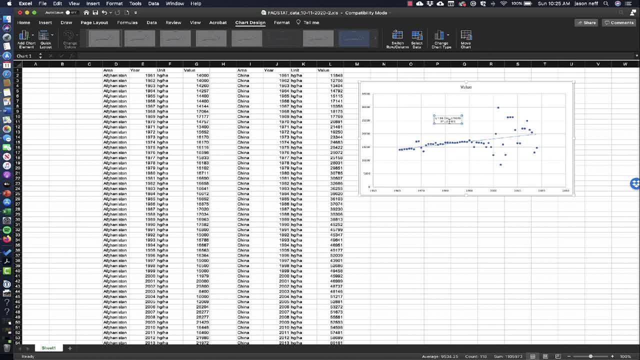 correctly. Make sure you're working in the application version of Excel and not the online version, Otherwise you won't have access to the trend line function. If you do all that, you should be able to work through this pretty quickly and you can start making the interesting. 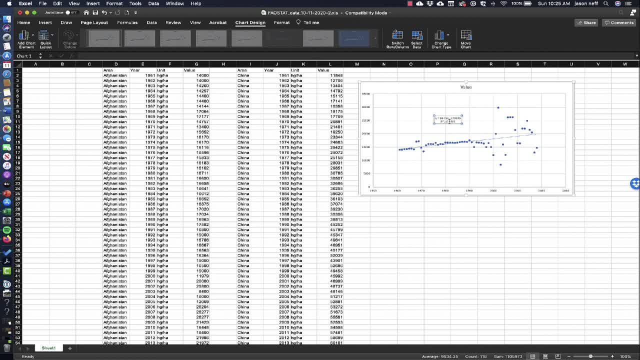 comparisons to see how yields have changed over time and also to see how the yields are different between countries. All right, good luck. 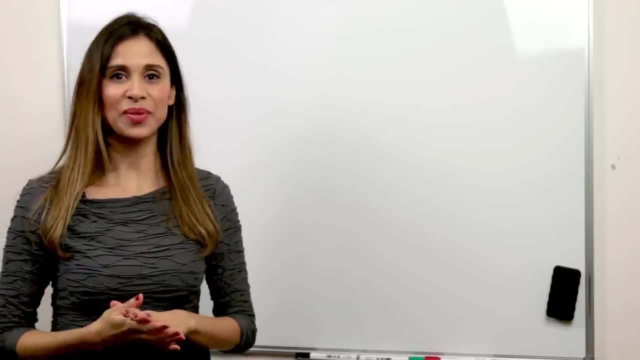 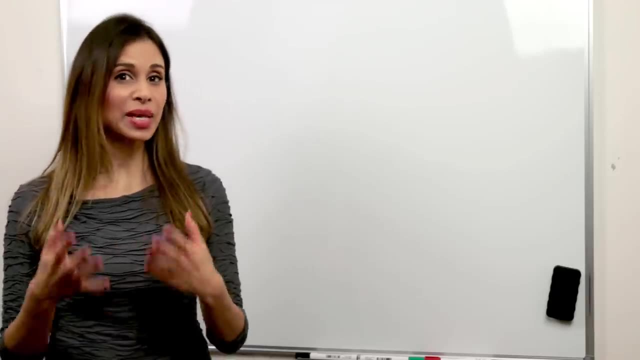 Today, let's take a look at calculating percentages in Excel. We're going to take a look at the formula you need to calculate percentage change and we're going to do it in a way that's going to help you remember it If you're working as a financial analyst, creating reports. this 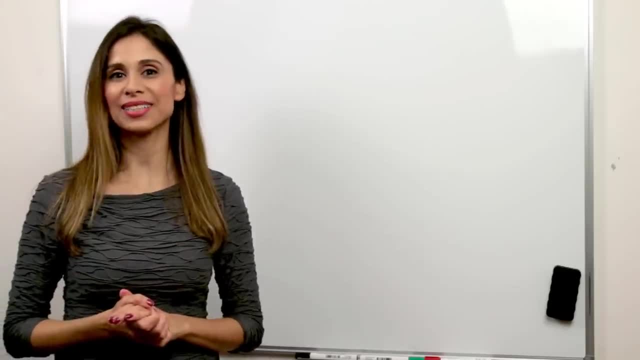 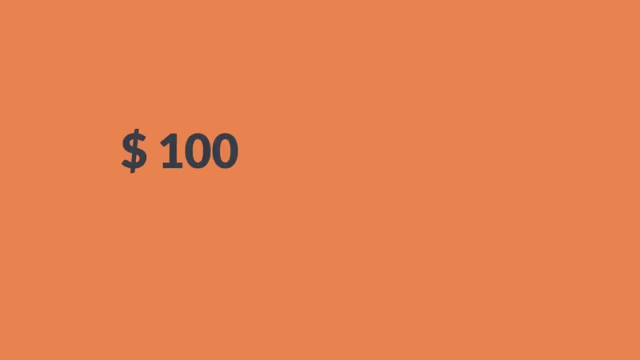 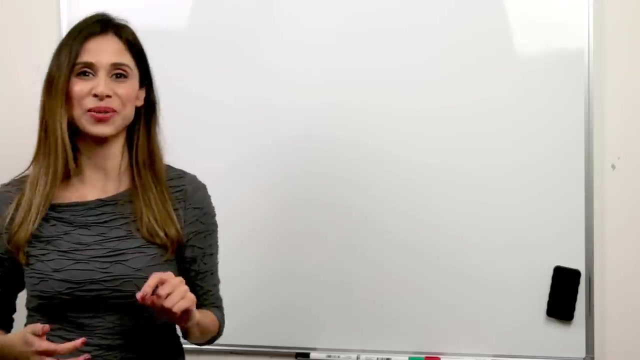 is a formula you need to get right. We're also going to take a look at how we can do calculations that involve percentage increase or decrease. So, for example, we have a price. We want to increase price by 15%. What's going to be our end price? Let's get to it. 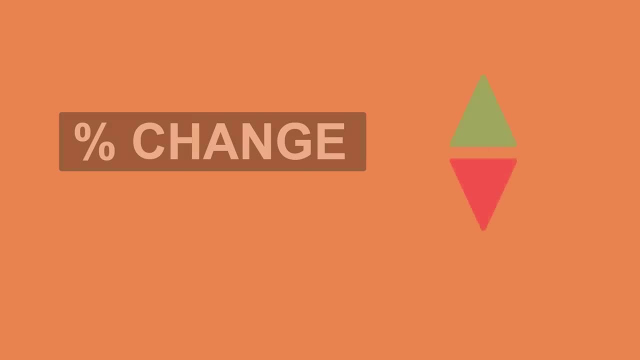 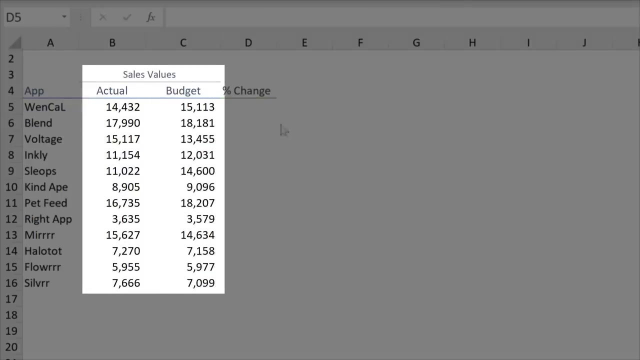 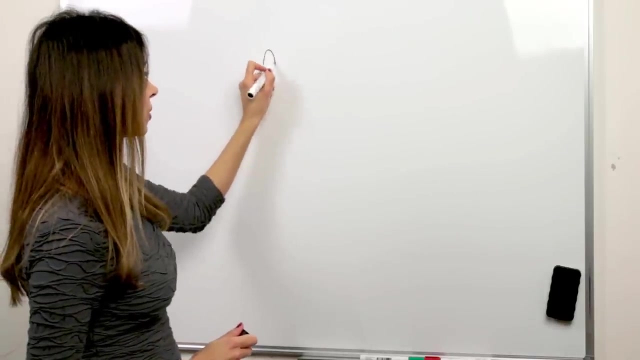 First off, let's take a look at calculating percentage change. Assume your boss gives you an Excel file that contains actual sales data and budget sales. Your task is to calculate percentage change. Let's take this to the board. So you have actual and you have budget. 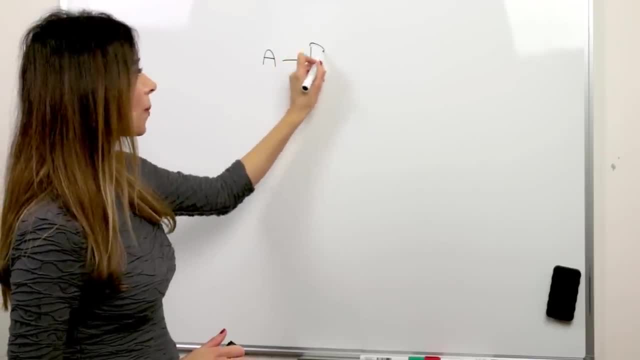 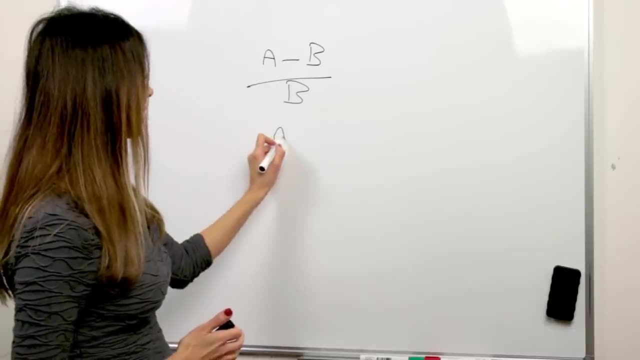 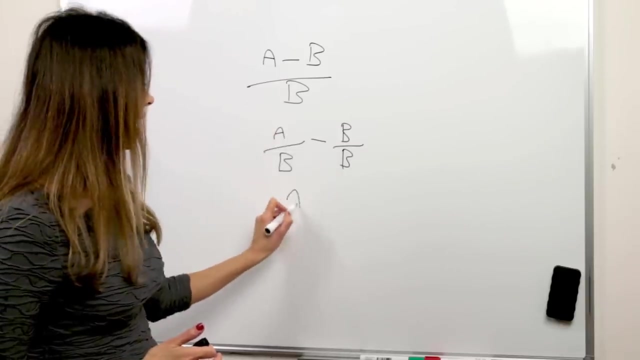 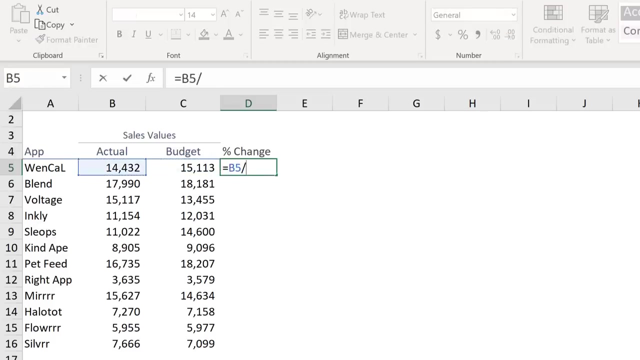 To calculate the difference, you're going to do actual minus the actual Minus budget divided by budget. An alternate way of writing this formula is actual divided by budget minus budget divided by budget, which turns into actual divided by budget minus one. Now it's all clear, right? So our formula is actual divided by budget minus. 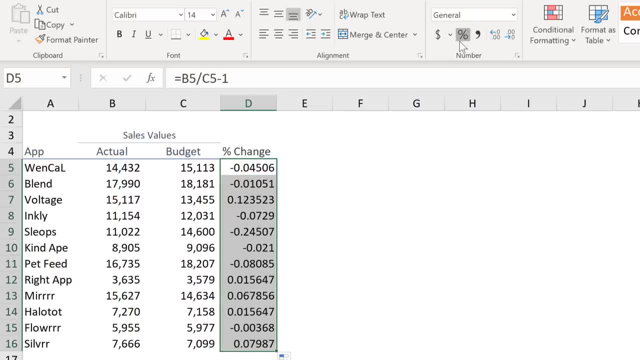 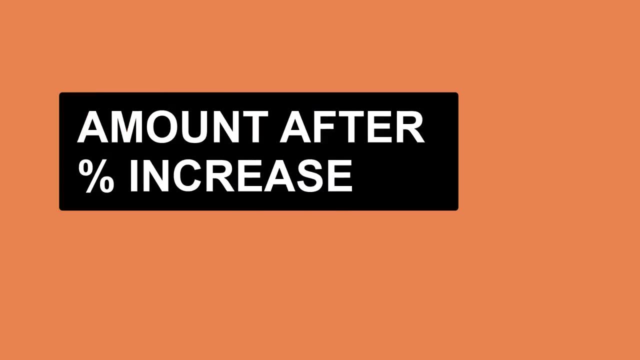 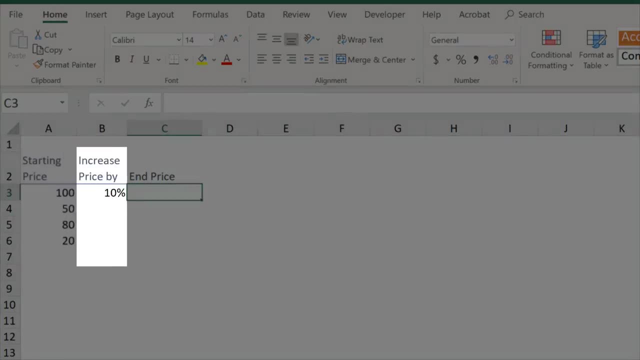 one Double click on the bottom right side and send the formula down. Now let's move on to calculating percentage increase or decrease. Our starting point is in column A. We want to increase the price by the percentage we see in column B and